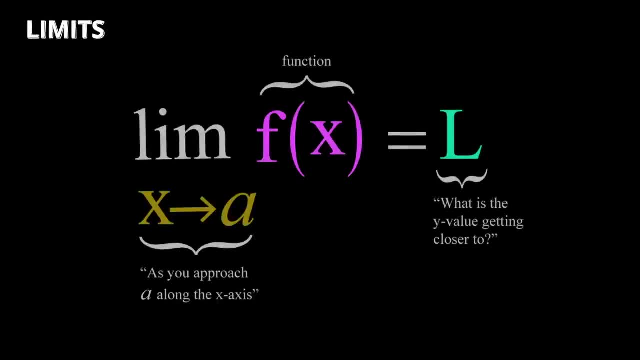 The general expression of limits is this. It is read as: the limit of f as x approaches a is the value l. These limits are evaluated using the general expression of limits. The general expression of limits is this: The general expression of limits is this. It is read as: the limit of f as x approaches a is the value l. 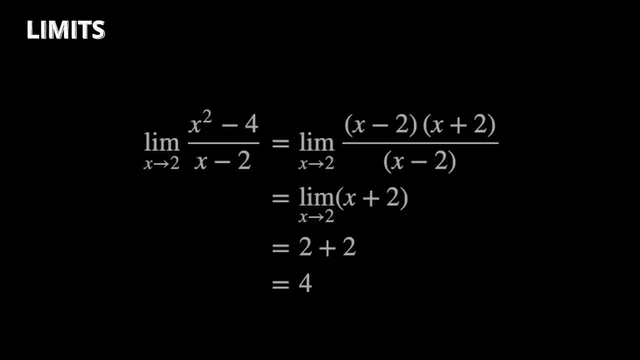 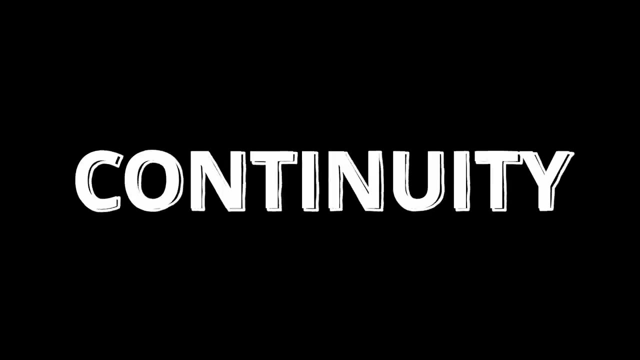 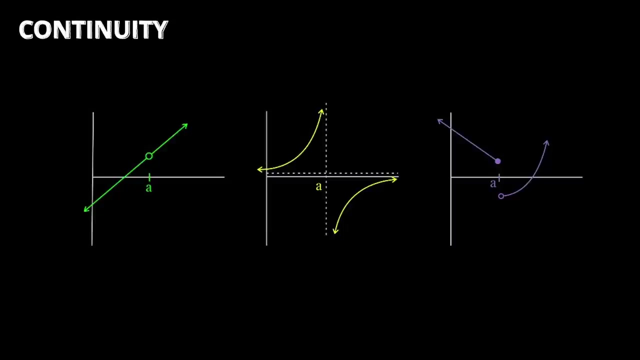 Usually by substitution or simplification. then substitution if the limit is initially indeterminate. Continuity: Sometimes, if these limits diverge or don't exist, discontinuities are made in our graph. There are three types of these discontinuities: The whole discontinuity, which looks like you. 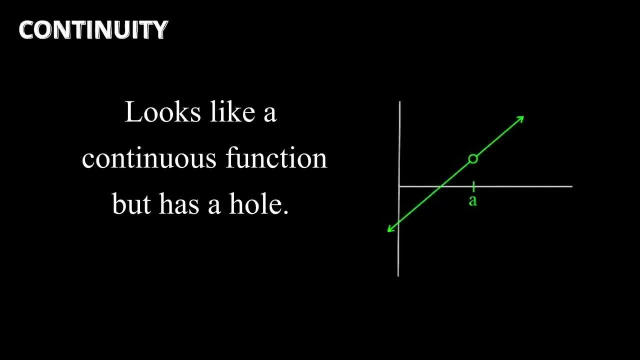 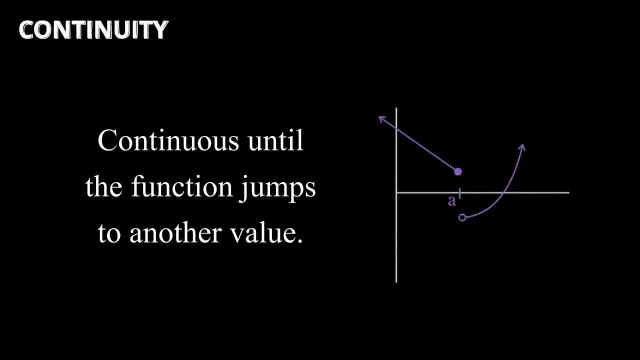 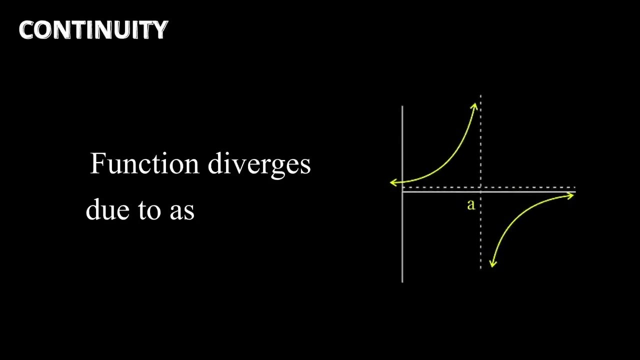 have a continuous graph, except for in one little point or whole, The jump discontinuity, which is continuous until a certain point, where the function jumps to another value and continues from there. Then you have the infinite discontinuity where asymptotes force the function to diverge. Functions are considered continuous at a point as long as they are defined. 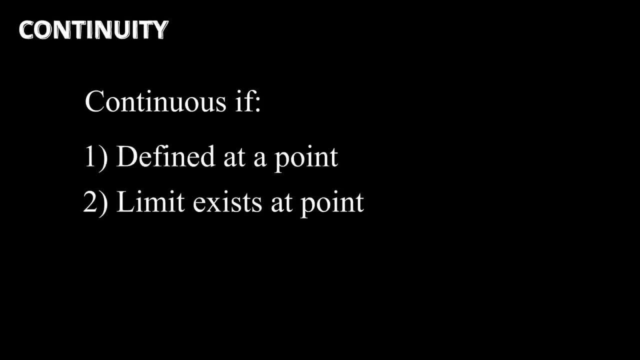 at the point. the limit exists at the point and the value of the function is the same as the value of the limit at the point. This is called the continuous discontinuity. The function is considered continuous at the point. Derivatives: Derivatives are what we use in calculus to observe the rate. 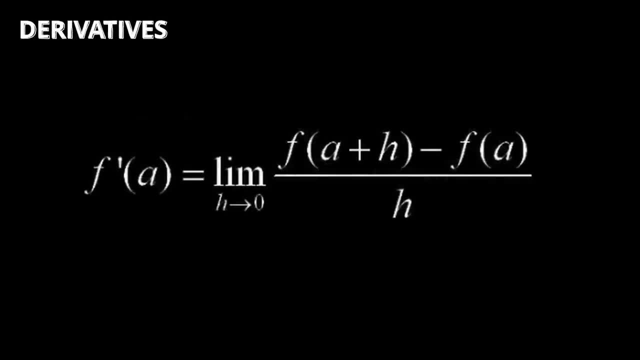 of change of functions. This is especially useful since it allows us to analyze the instantaneous slope of functions at certain points, as opposed to what we used to do before calculus, which was simply taking average slope. Derivatives are usually denoted using the Lagrange and Leibniz. 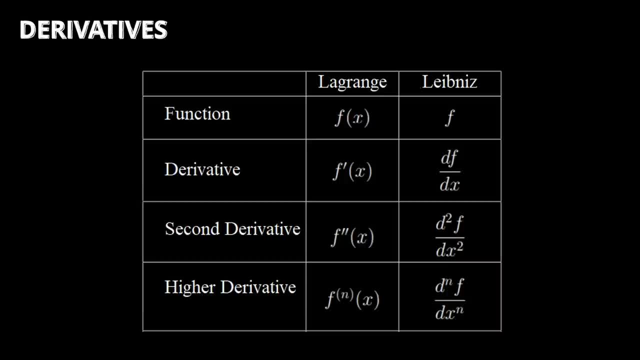 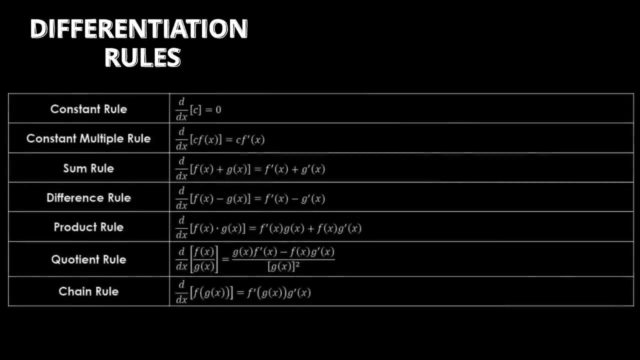 notation like this: You can even take higher order derivatives, which is just taking the derivative of the derivative to get the slope of the slope. Differentiation rules: These are the rules we use to actually evaluate and take derivatives. These are the constant rule.